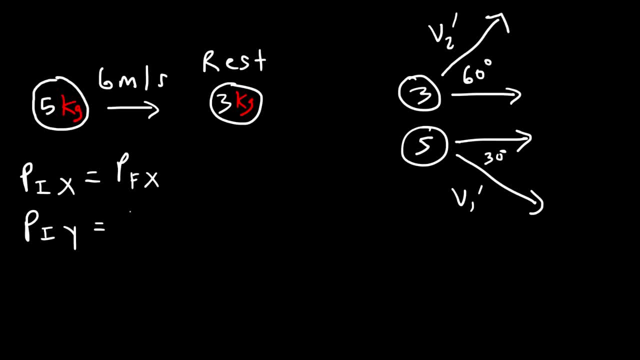 And the momentum in the y-direction must be conserved. So this is going to be v2x and this is v2y prime. And here we have v1x And this is going to be v1y prime. So feel free to try this problem. 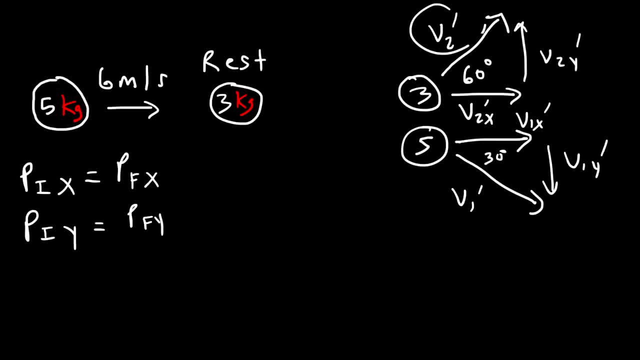 Go ahead and pause the video. Calculate the final velocities of the 5 kilogram ball and the 3 kilogram ball after the collision. So let's start with the momentum in the x-direction. So let's start with this equation: M1v1x plus M2v2x. 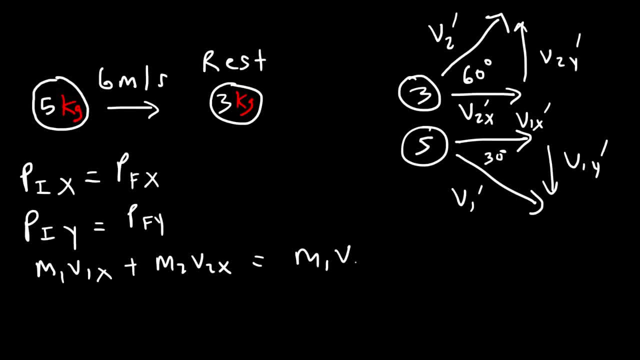 M1v2x is equal to M1v1x prime plus M2v2x prime. So v1x is the initial velocity of the 5 kilogram ball in the x-direction. V1x prime is the final velocity of the first ball, the 5 kilogram ball, in the x-direction. 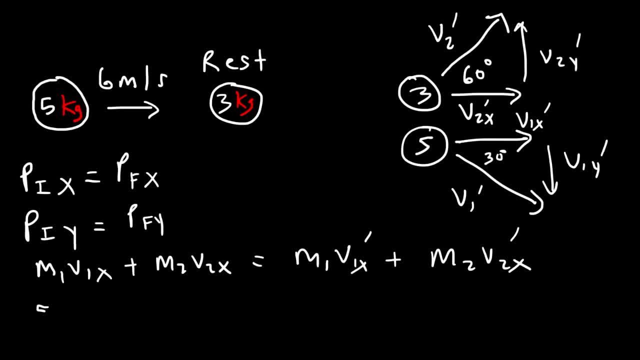 So you understand what these things represent. So M1 is 5.. V1x is 6 because it was moving in the x-direction. Now the second ball is at rest. M1 is still 5.. Now what is v1x prime? 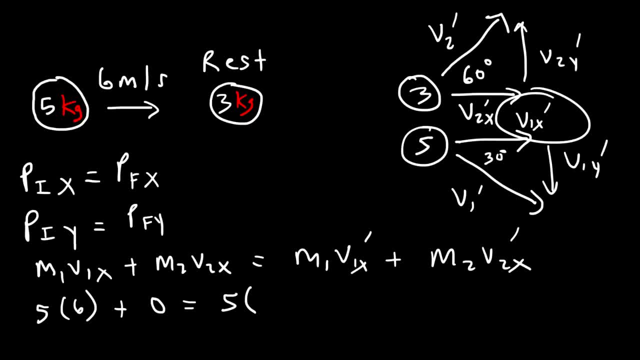 So that represents this term. here It is the x-component of this value. So it's going to be v1 prime times cosine theta. So it's v1 prime cosine Of negative 30 degrees. It's negative 30 because it's below the x-axis. 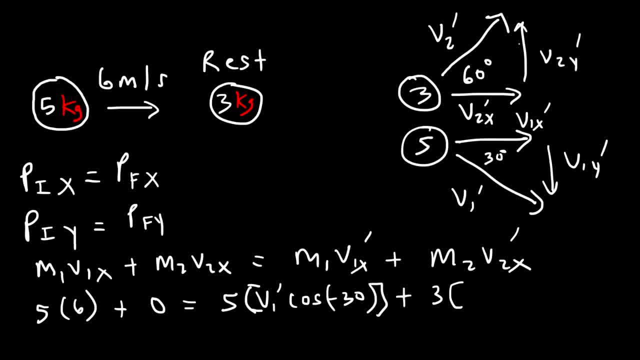 M2, the second mass is 3 kilograms And v2x prime. that's going to be v2 times cosine of this angle, which is 60 degrees. So 5 times 6 is 30. And then 5.. 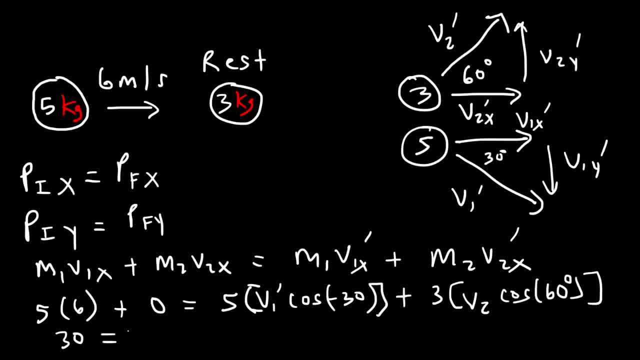 times cosine of negative 30 degrees is 4.33 times V1 prime and 3 times cosine 60, that's going to be 1.5 times V2 prime. So let me get rid of some stuff. So I'm going to write this equation on top. 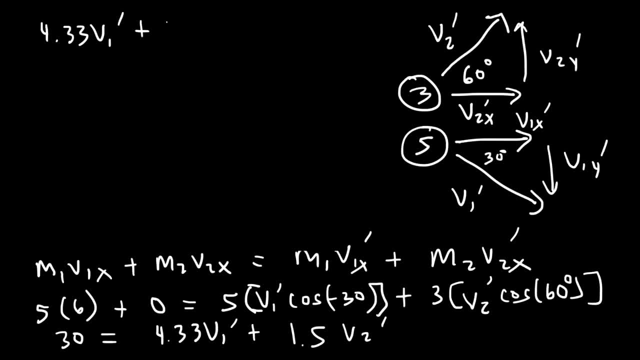 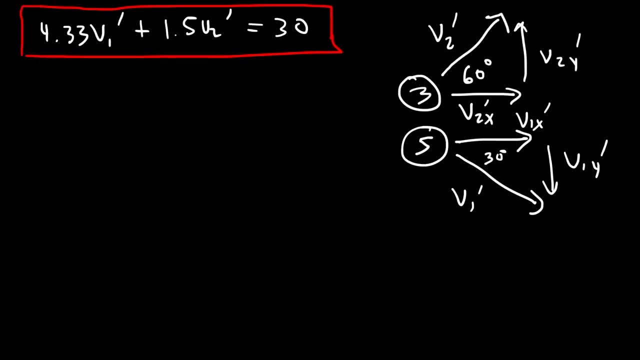 So it's 4.33 V1 prime plus 1.5 V2 prime equals 30.. So let's save that equation. So now let's focus on the momentum in the Y direction. So M1 V1Y plus M2.. 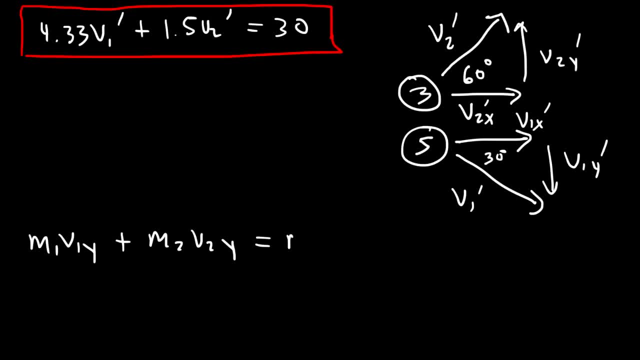 So M1 V2Y is equal to M1 V1Y prime plus M2 V2Y prime. So the 5 kilogram ball was moving at 6 meters per second. It was moving in the X direction, so there was no Y component. 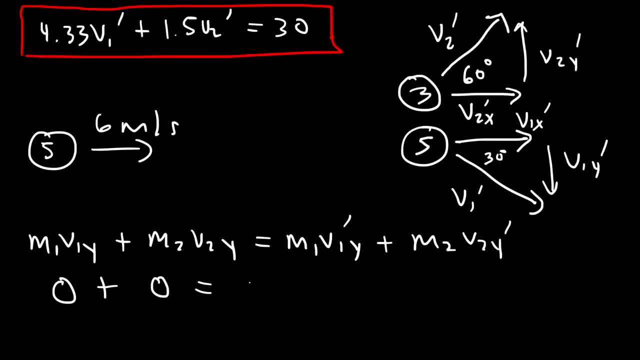 And the second ball was at rest, so it had no momentum, And this is going to equal 5 times Now: V1 prime, V1, prime, final. That's going to be that term, which is V1, prime times, sine of the angle. 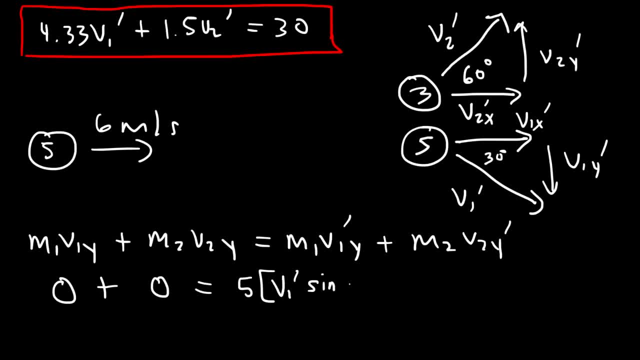 So this is going to be V1 prime times sine of negative 30.. And then the second mass is 3.. So V2Y prime is going to be V2 prime multiplied by sine of this angle 60. So 5 times sine of negative 30.. 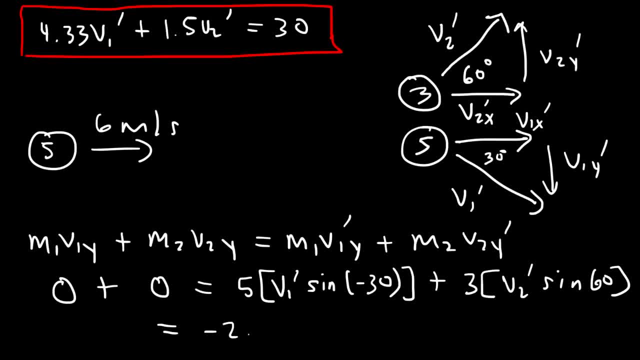 That's negative 2.5 times V1 prime, And then 3 sine 60. That's going to be positive 2.5981 times V2 prime And this is equal to 0. So I'm going to take this term and move it to this side. 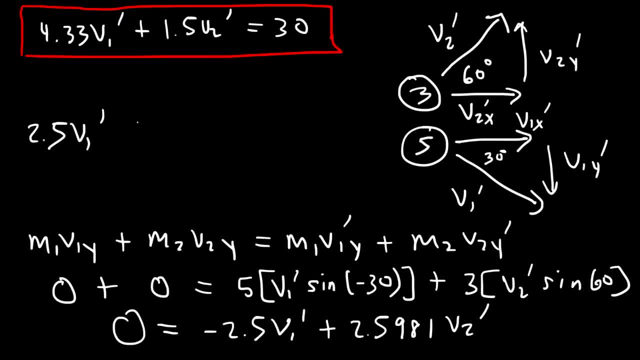 So what I now have is 2.5 V1 prime is equal to 2.5981 V2 prime. So to solve V2 prime, I'm going to divide both sides by this number, So 2.5 divided by 2.5981. 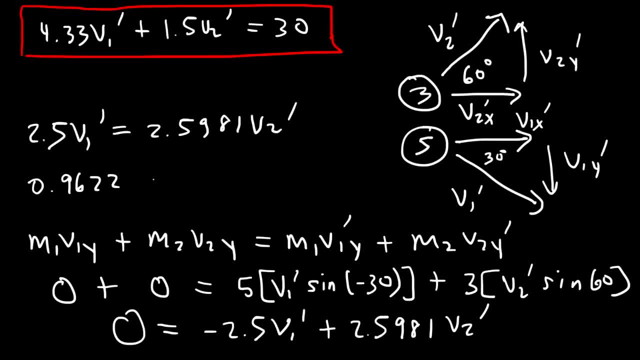 That's 0.9622 times V1 prime. So that's equal to V2 prime, Which I'm going to rewrite it here. So that's the second equation that we need. So with these two equations we could solve for the two missing variables. 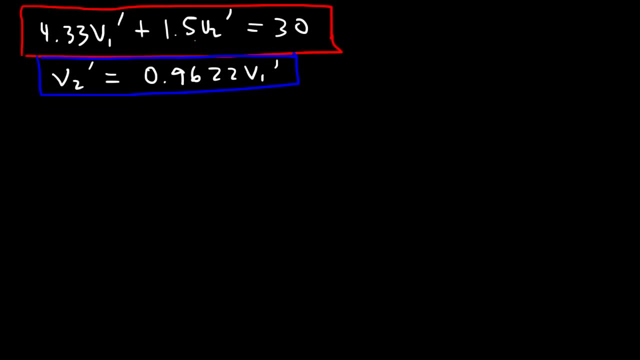 So now all we need to do is solve by substitution. We need to replace V2 prime with 0.9622 V1 prime, So this is going to be 4.33 V1 prime plus 1.5 times 0.9622 V1 prime. 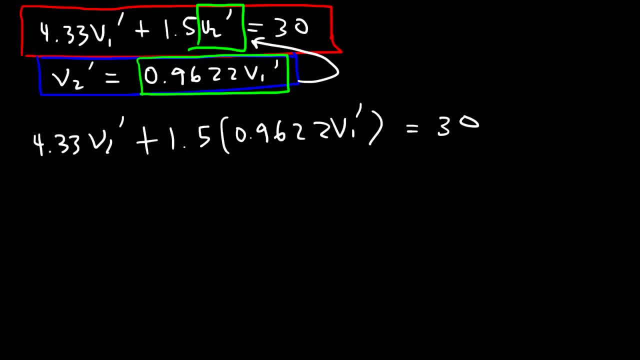 And that's equal to 30.. So let's multiply 1.5 by 0.9622.. So you should get 1.4433 V1 prime. So now let's combine like terms, So 1.4433 plus 4.33.. 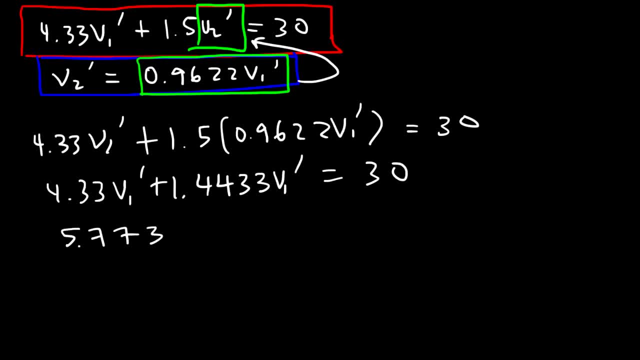 That's going to be 5.7733 V1 prime, And that's equal to 30.. So V1 prime is going to be 30.. Divided by 30. That's equal to 5.7733.. And so you should get 5.196 meters per second for the final velocity of the 5 kilogram ball. 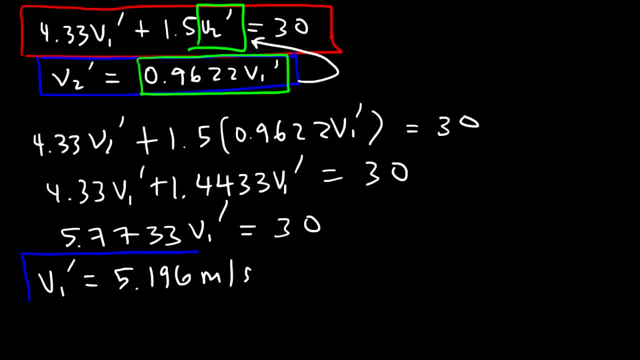 That's the first one. So now with this answer we could take it and plug it into this equation to calculate the velocity of the second ball. So V2 prime That's going to be 0.9622.. Multiplied by 5.196..